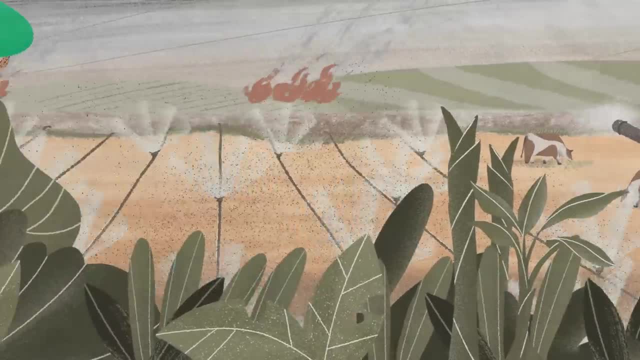 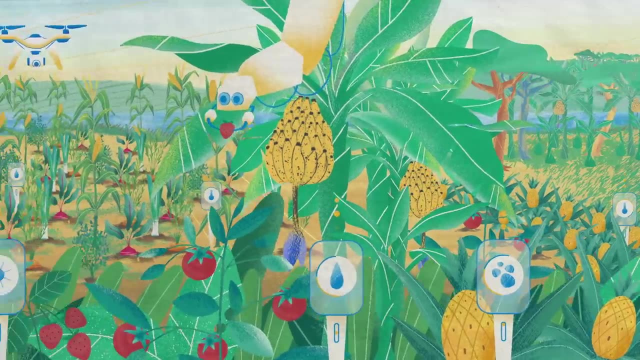 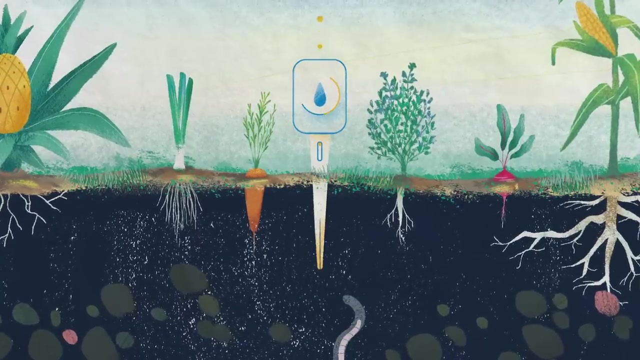 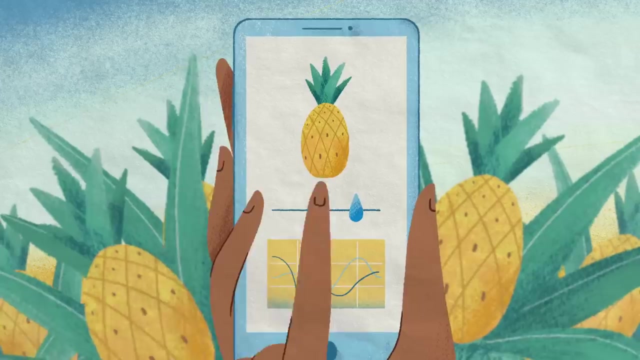 wildlife and emitting huge amounts of greenhouse gases in the process. This approach aims to correct that damage. Meanwhile, moving among the crops, teams of field robots apply fertilizer in targeted doses Inside the soil. hundreds of sensors gather data on nutrients and water levels. This information reduces unnecessary water use. 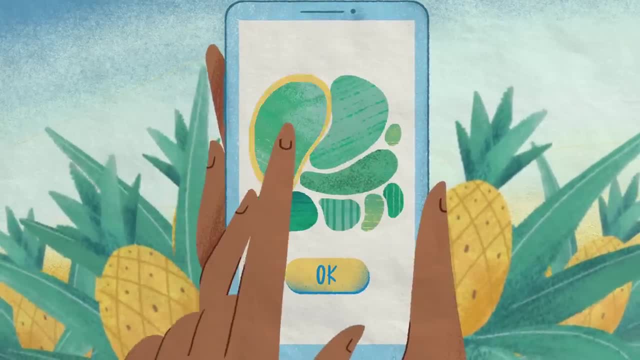 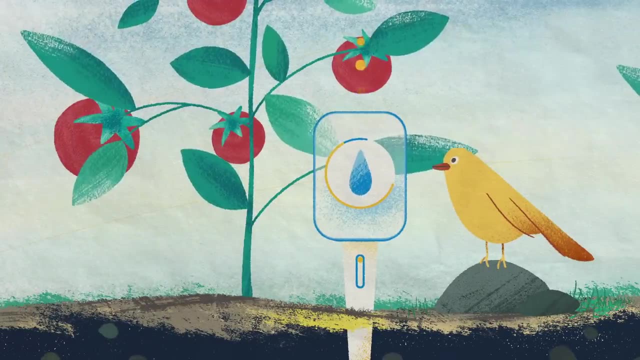 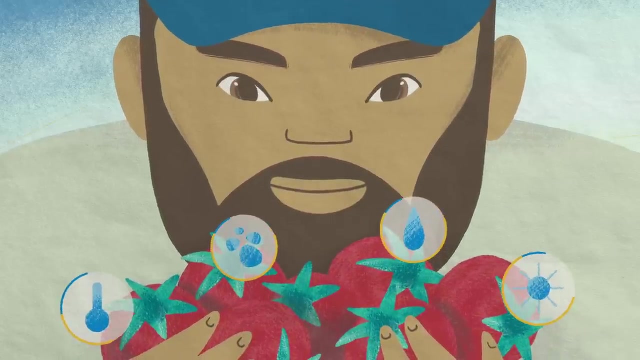 and tells farmers where they should apply more and less fertilizer instead of causing pollution by showering it across the whole farm. But the farms of the future won't be all sensors and robots. These technologies are designed to help us produce food in a way that works with the environment. 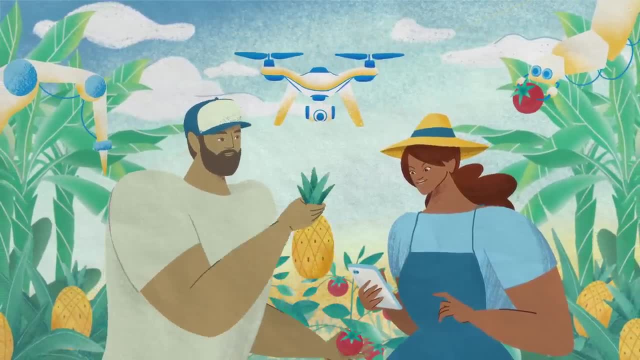 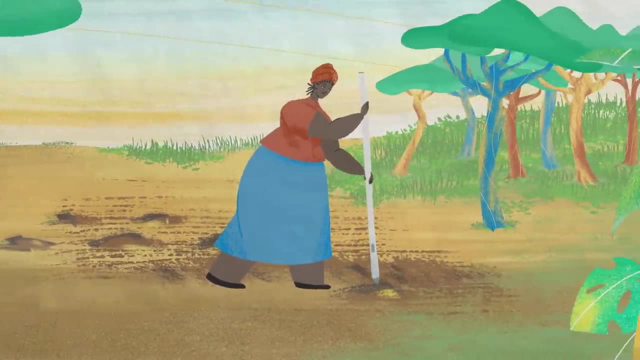 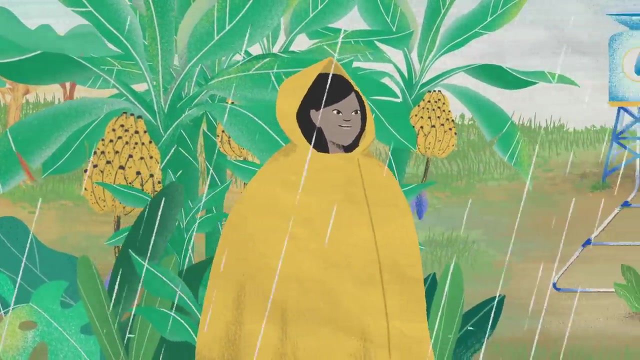 rather than against it, taking into account the nuances of local ecosystems. Lower-cost agricultural practices can also serve those same goals and are much more accessible to many farmers. In fact, many such practices are already in use today and stand to have an. 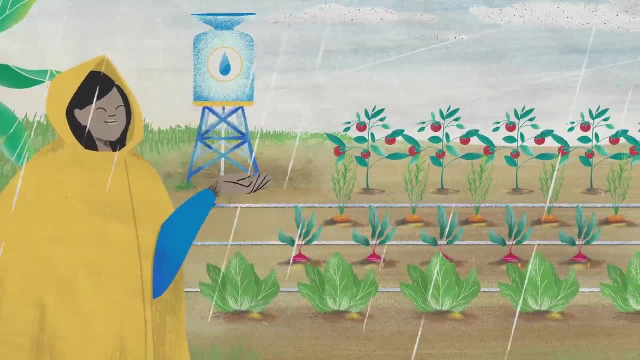 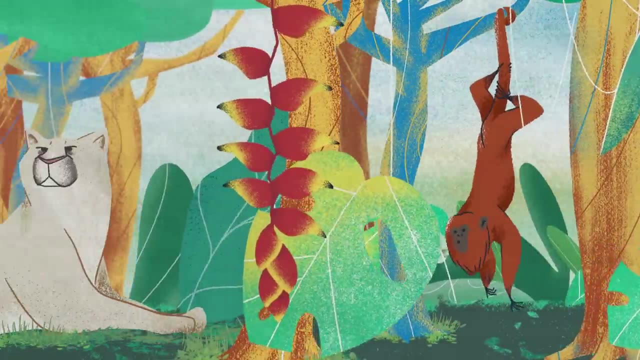 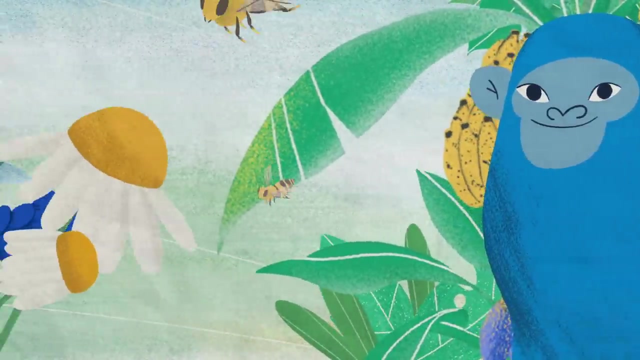 increasingly large impact on the future of agriculture and the future of the environment. In Costa Rica, farmers have intertwined farmland with tropical habitat so successfully that they've significantly contributed to doubling the country's forest cover. This provides food and habitat for wildlife, as well as natural pollination. 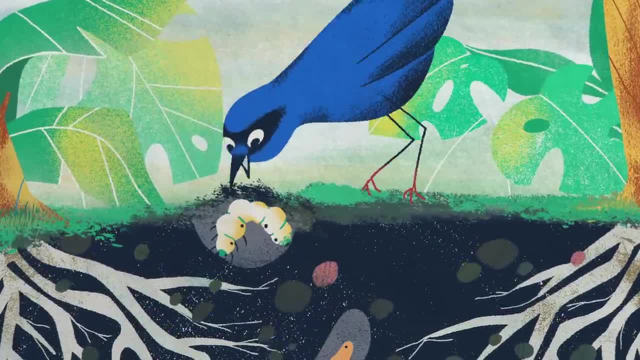 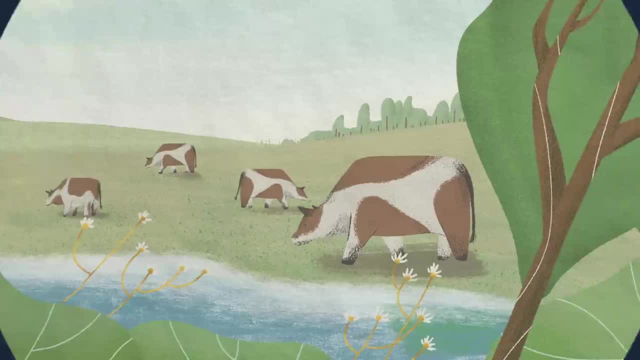 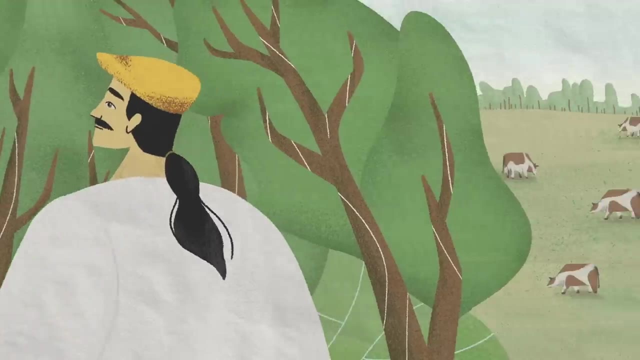 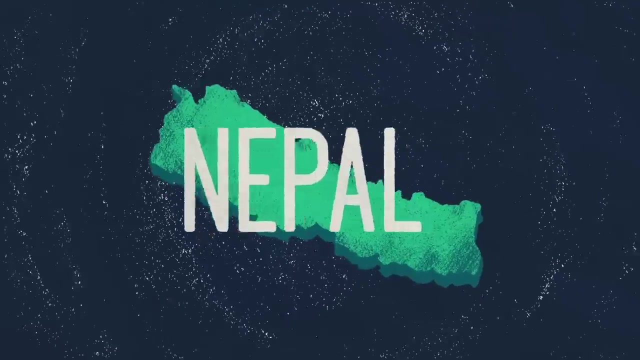 and pest control from the birds and insects these farms attract, producing food while restoring the planet. In the United States, ranchers are raising cattle on grasslands composed of native species, generating a valuable protein source, using production methods that store carbon and protect biodiversity. In Bangladesh, Cambodia and Nepal, new approaches to rice. 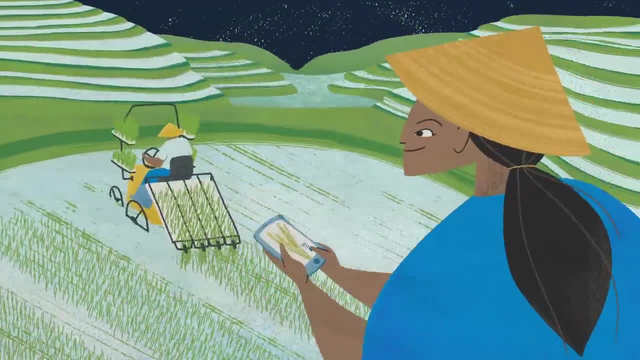 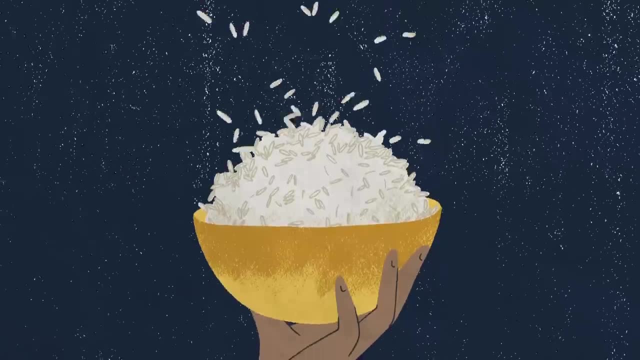 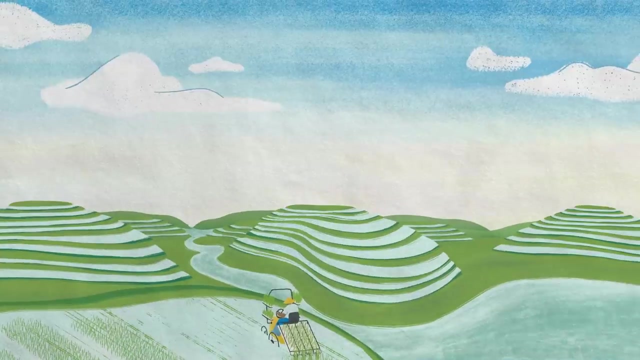 production may dramatically decrease greenhouse gas emissions in the future. Rice is a staple food for 3 billion people and the main source of livelihood for millions of households. More than 90% of rice is grown in flooded paddies. These paddies use a lot of water and release 11% of annual methane emissions. 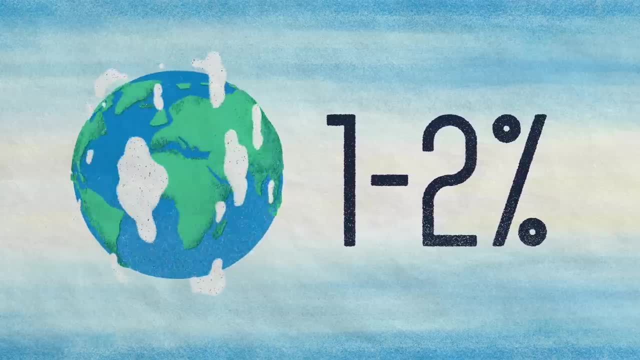 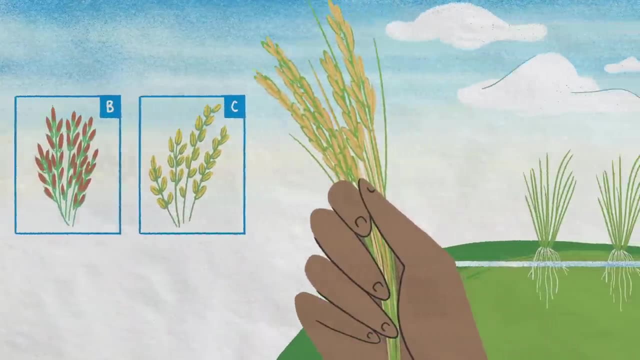 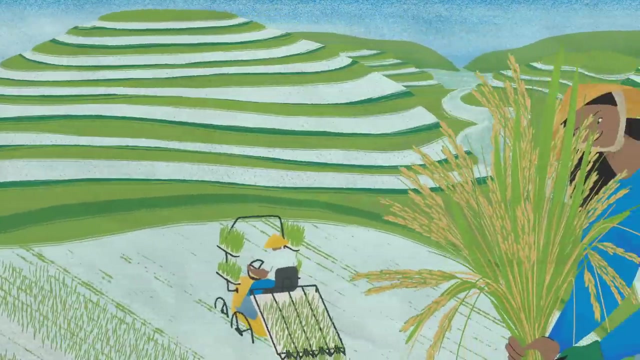 which accounts for 1-2% of total annual greenhouse gas emissions globally. By experimenting with new strains of rice, irrigating less and adopting less labor-intensive ways of planting seeds, farmers in these countries have already increased their incomes and crop yields while cutting down on greenhouse gas. 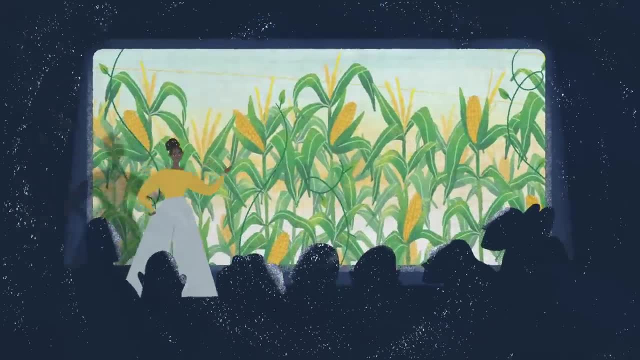 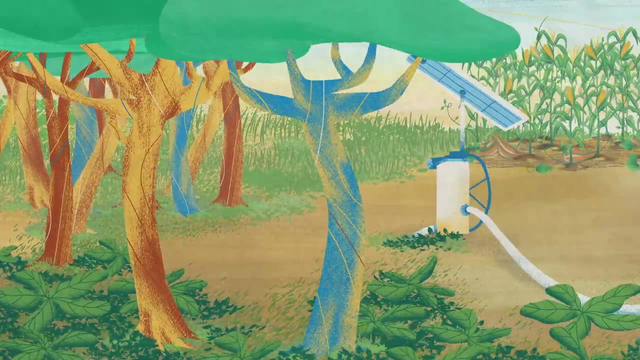 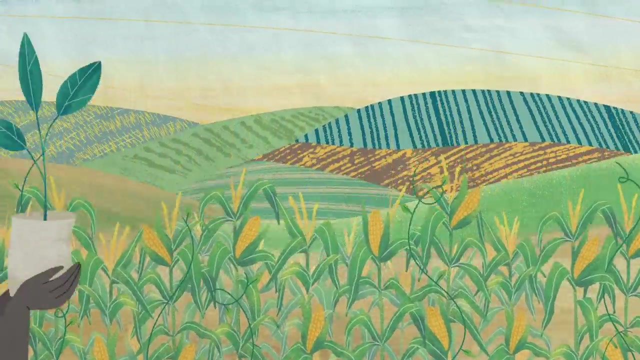 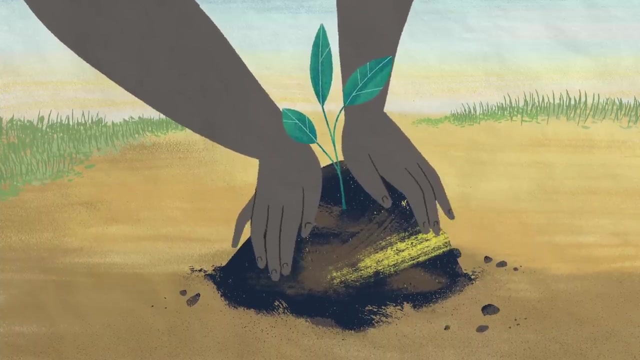 emissions. In Zambia, numerous organizations are investing in locally specific methods to improve crop production, reduce forest loss and improve livelihoods for local farmers. These efforts are projected to increase crop yield by almost a quarter over the next few decades. If combined with methods to combat deforestation in the region, they could move the country toward a resilient 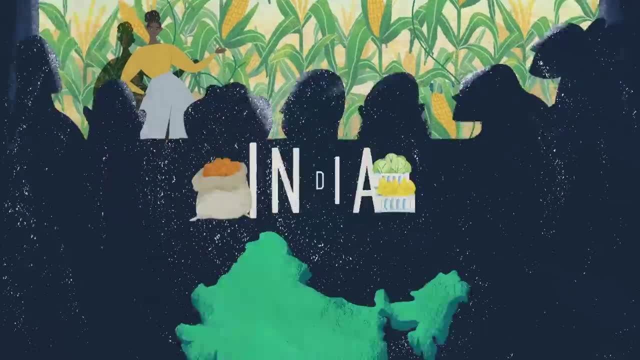 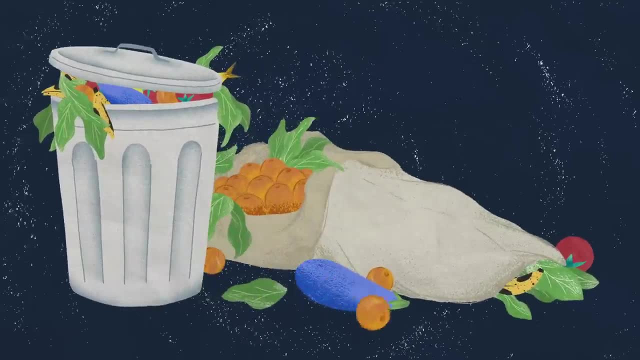 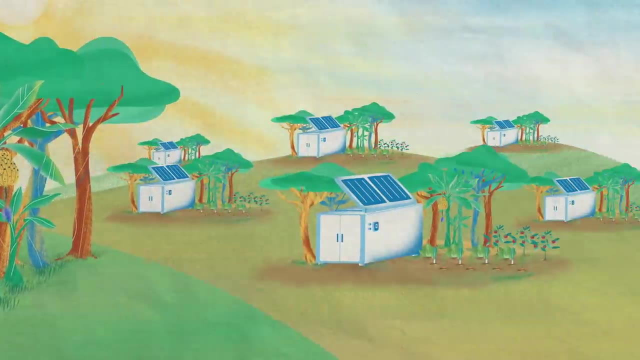 climate-focused agricultural sector, And in India, where up to 40% of post-harvest food is lost or wasted due to poor infrastructure, farmers have already started to implement solar-powered cold storage capsules that help thousands of rural farmers preserve their produce and become a viable part of the supply chain. 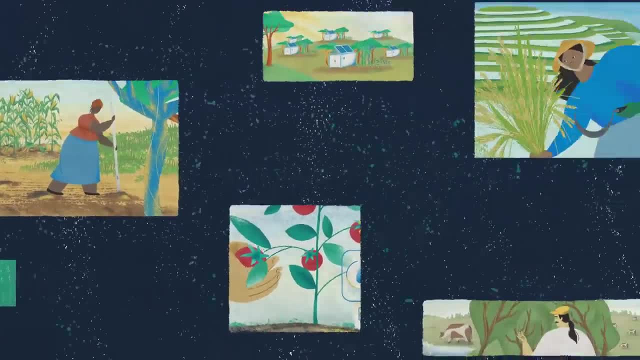 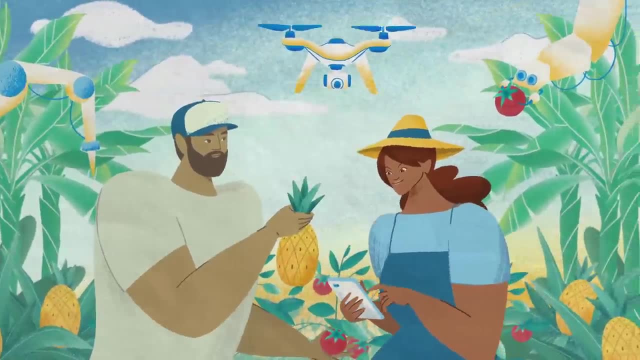 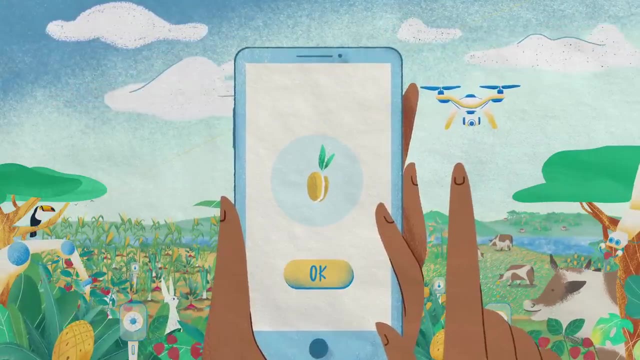 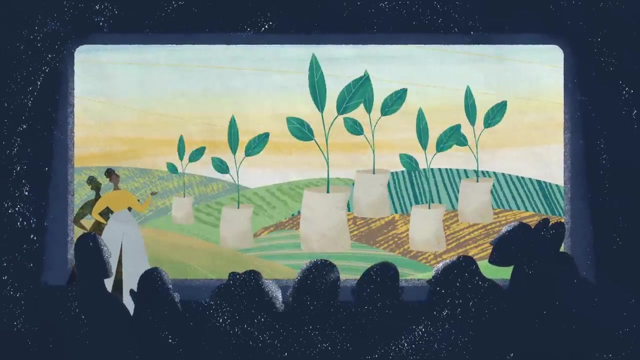 The system calls for talks about these methods to be implemented from high-tech top ten extension to 96%oph. Goodbye, Bye. amplify climate and conservation-oriented approaches to farming, and large producers will need to invest in implementing these technologies. Meanwhile, we'll have to expand access to the lower-cost methods for smaller-scale farmers. 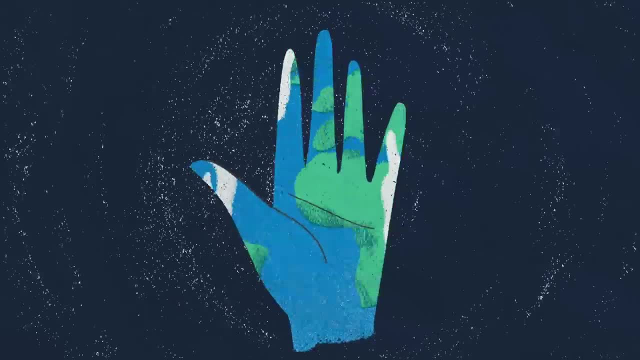 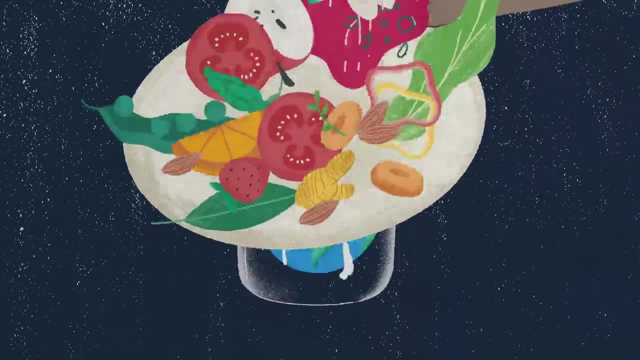 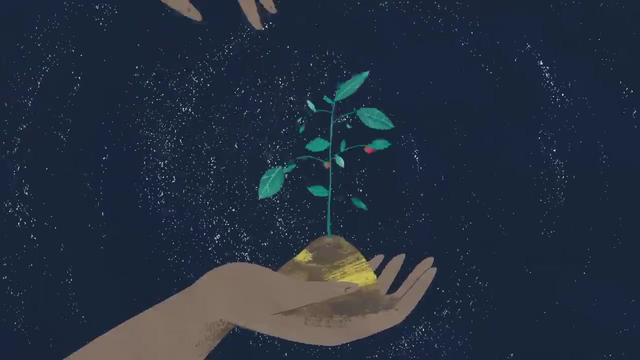 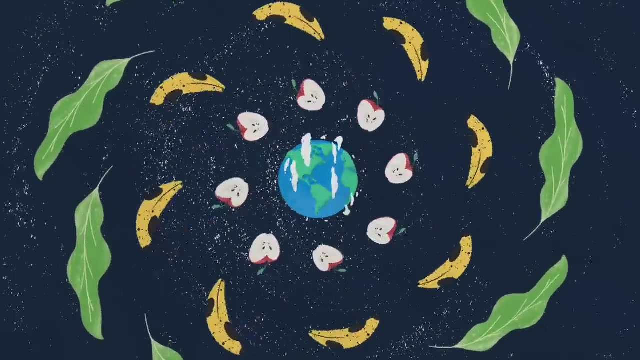 This vision of future farming will also require a global shift toward more plant-based diets and huge reductions in food loss and waste, both of which will reduce pressure on the land and allow farmers to do more with what they have available. If we optimize food production both on land and sea, we can feed humanity within the environmental 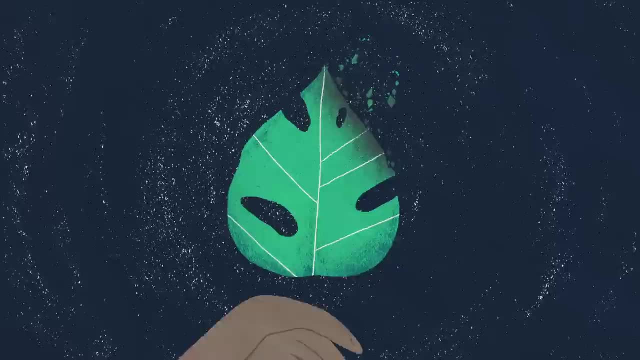 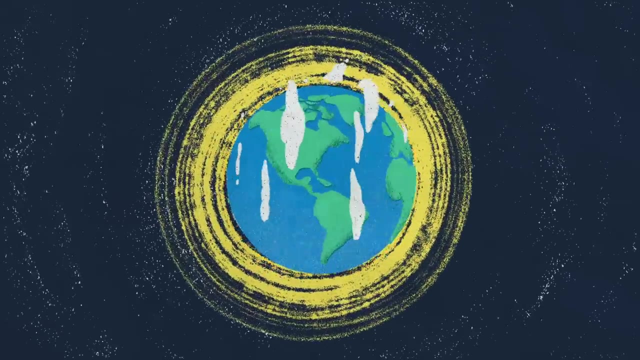 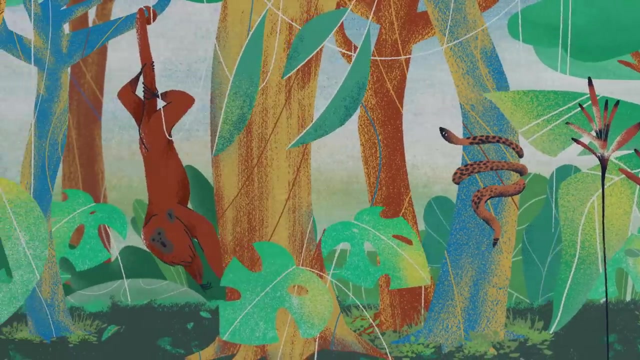 limits of the earth. But there's a very small margin of error and it will take unprecedented global cooperation and coordination of the agricultural lands we have today. An agricultural revolution can start with a change. Join Countdown, a global initiative bringing together scientists, activists, urban planners.